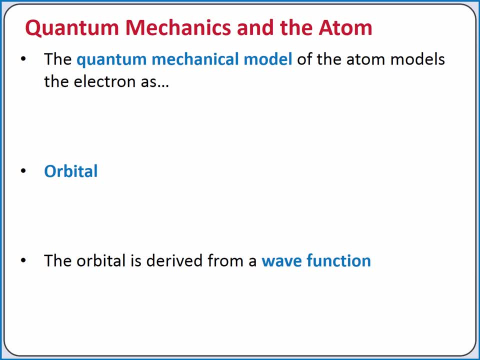 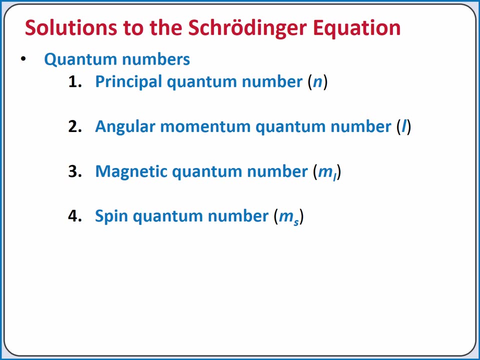 Based on each of these solutions to the Schrodinger equation, we can create an orbital, which is the volume that encompasses 90% of the probability of finding an electron. Each orbital is designated by three quantum numbers: the principal quantum number, angular momentum quantum number and magnetic quantum number. 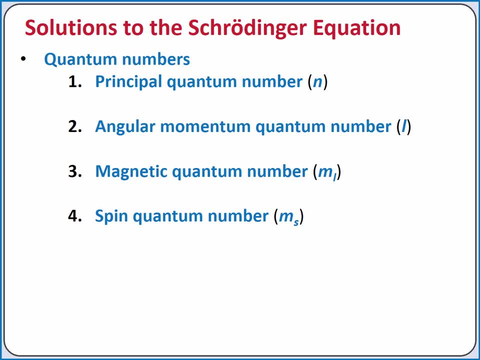 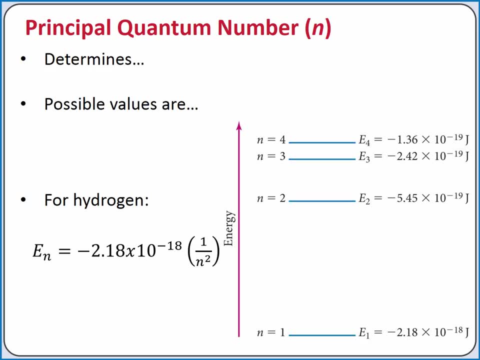 A fourth quantum number. the spin quantum number designates an electron within it. Our principal quantum number n determines the size and energy of an orbital. The possible values are integers 1,, 2,, 3,, 4,, etc. 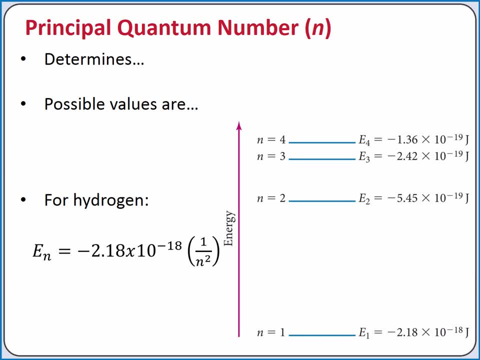 As the value of n increases, the orbital has a higher energy and the electrons within the orbital are generally farther away from the nucleus For the hydrogen atom. we can calculate the energy of the electron within the orbital. To calculate the energy of each orbital based on the equation: 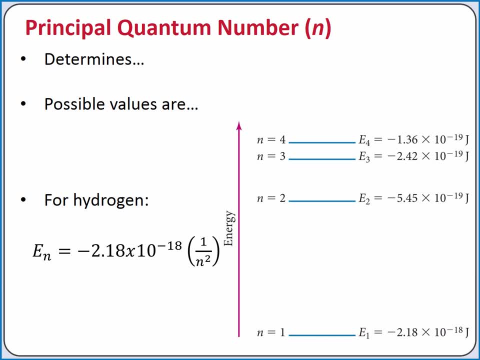 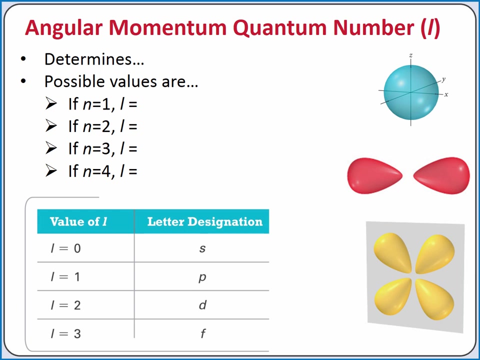 energy equals negative 2.18 times 10 to the negative 18th power times the quantity 1 divided by n. squared With multi-electron atoms, the calculation becomes more complicated. The angular momentum quantum number L determines the shape of an orbital. 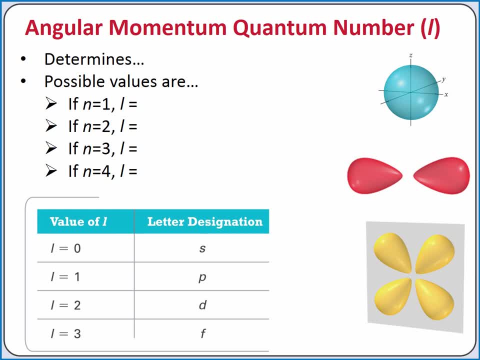 The possible values are integers from 0 to n minus 1.. So if n equals 1,, the only possible value of L is 0.. If n equals 2,, the possible values are 0 or 1.. If n equals 3,, the possible values are 0,, 1, or 2.. 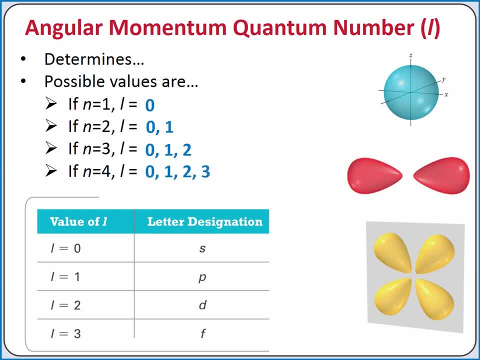 And if n equals 4,, the possible values are 0,, 1,, 2, or 3.. There are also letter designations for each variable. L equals 0 is also called S, and it corresponds to the shape of the sphere shown in blue. 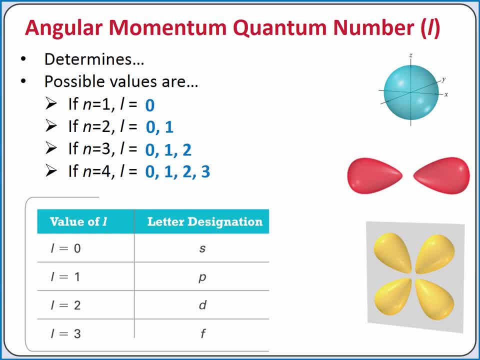 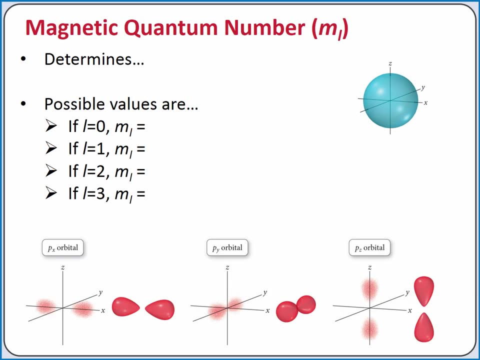 L equals 1 is P and corresponds to the red dual teardrop shape. L equals 2 is D and L equals 3 is F. The magnetic quantum number m sub L determines the orientation. Possible values of m sub L are integers from negative L to positive L, including 0.. 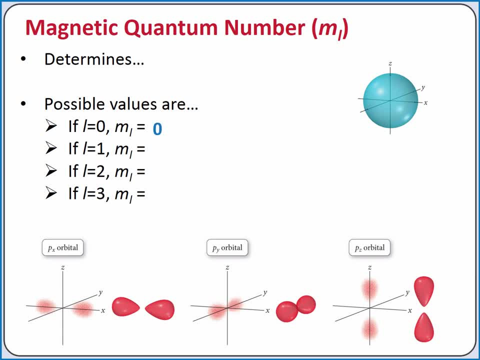 So if L equals 0,, the only possible value of m sub L is 0.. This means there is only one orientation for the S shape. If L equals 1, the possible values of m sub L are negative, 1,, 0, and positive 1.. 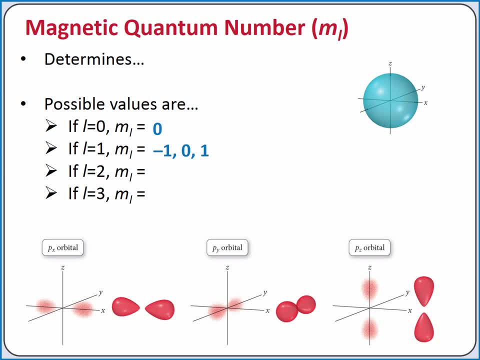 These three possible orientations of the P shape are centered on the X, Y and Z axes. When L equals 2,, there are five possible orientations for the D shape, corresponding to the numbers negative 2 through positive 2.. And when L equals 3,, there are seven possible orientations for the F shape. 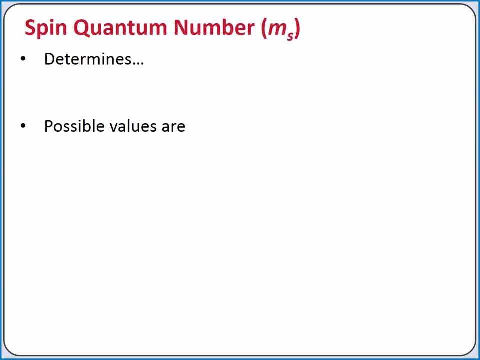 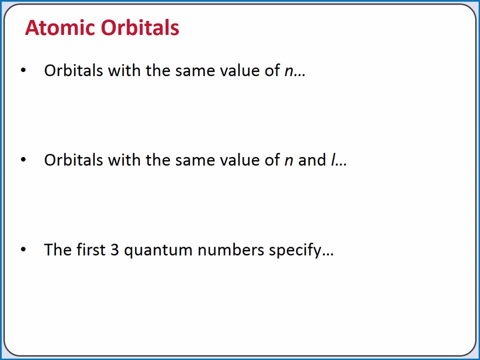 The spin quantum number determines the spin of the electron within the orbital. The possible values are positive 1 half and negative 1 half, So each orbital can hold two electrons. Orbitals with the same value of n are said to be in the same shell or principal level. 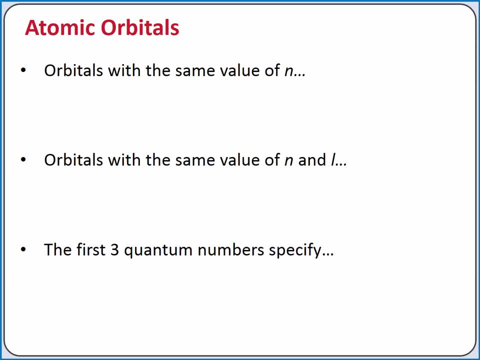 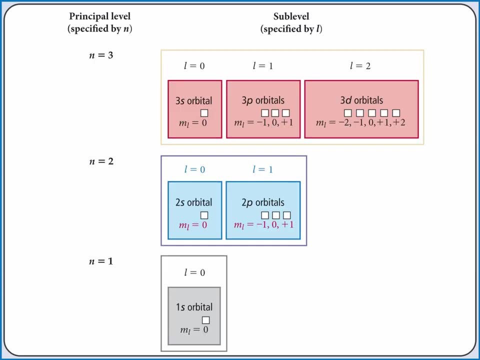 Orbitals with the same value of n and L are said to be in the same sub-shell or sub-level, And the first three quantum numbers specify a single orbital within the atom. We can apply our possible values for our quantum numbers to an atom. 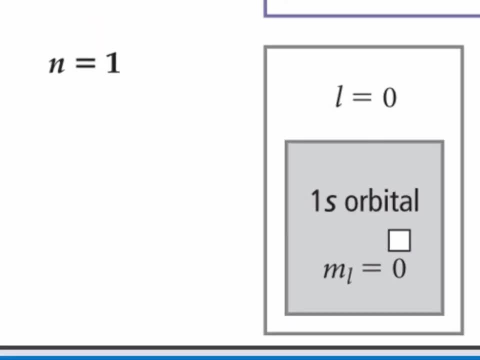 When n equals 1, the only possible value of L is 0.. This corresponds to the S shape. When L equals 0, the only value of m sub L is 0. So there is only one orbital in the 1S sub-shell. 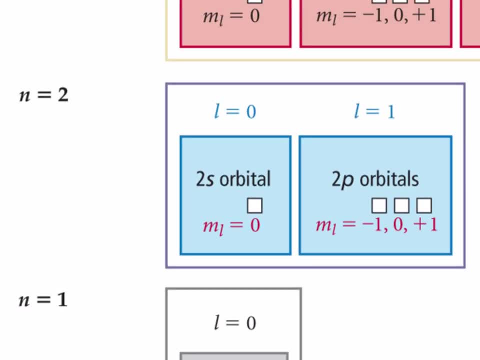 When n equals 2, the possible values of L are 0 or 1.. We have one orbital in the 2S sub-shell, but we have three orbitals in the 2P sub-shell, which corresponds to the three possible values of m sub L when L equals 1..